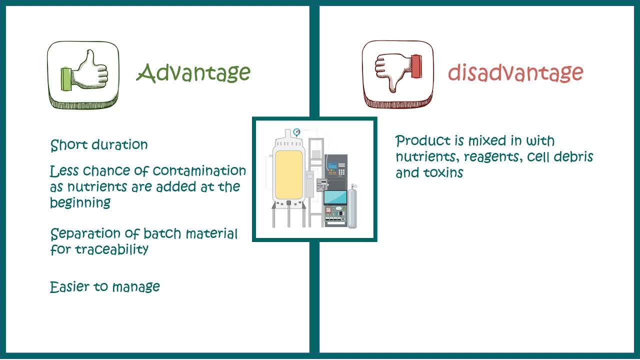 these kind of processes. but the problem is product is mixed with nutrients, reagents, cell debris and toxins which might affect the yield. and in industrial settings the yield is the biggest thing. right yield and the profit. next we are going to talk about the production time. so since after one run of 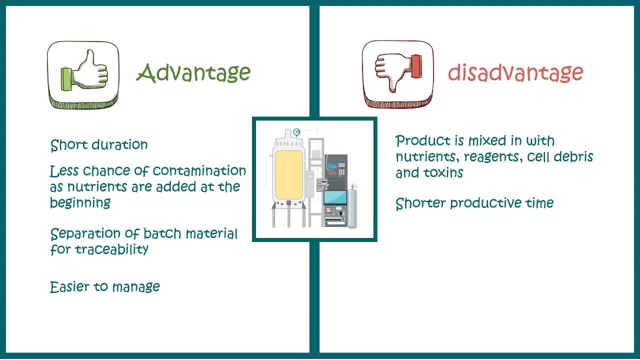 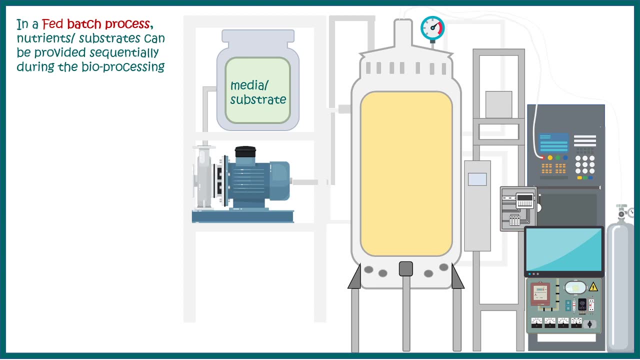 bioreactor, there would be some downtime. then the effective productive time is really low, so overall productivity of this process is not so high. a little bit modification in this batch process is known as fade batch process, where nutrients or substrates can be injected sequentially. so you begin with a partial 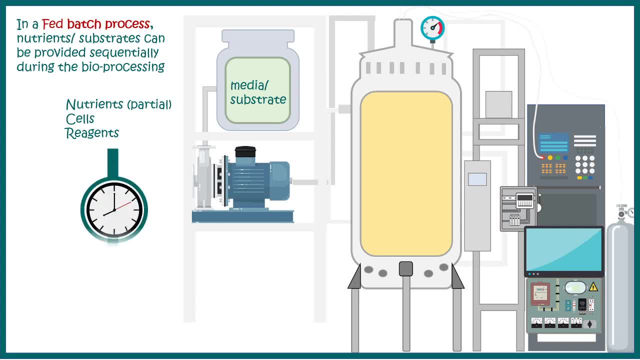 concentration of nutrient or media and eventually one can inject the nutrients or media throughout this process. Now this allows the harmful effect of high concentration of media at the beginning. Let's say the media might inhibit the growth kinetics of these cells. So this particular process can 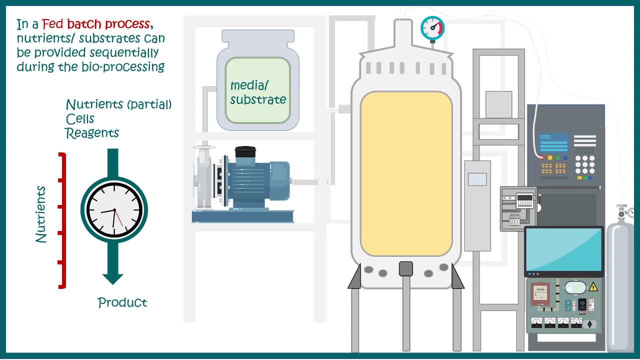 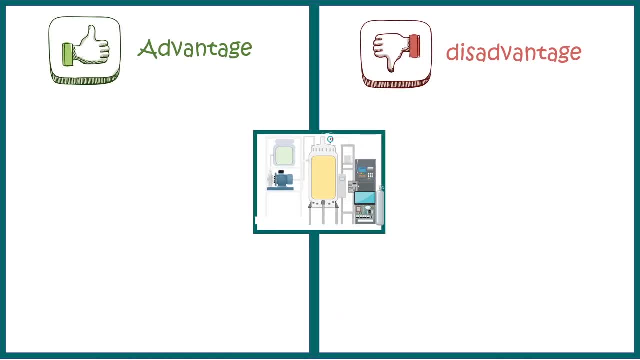 overcome those kind of drawbacks. Next we'll talk about the advantage and disadvantage of this process. Now this actually extends the cultures productive duration, So reactor downtime versus productive length is more in this case. It can be used to switch on genes and switch off genes in case of a specific. 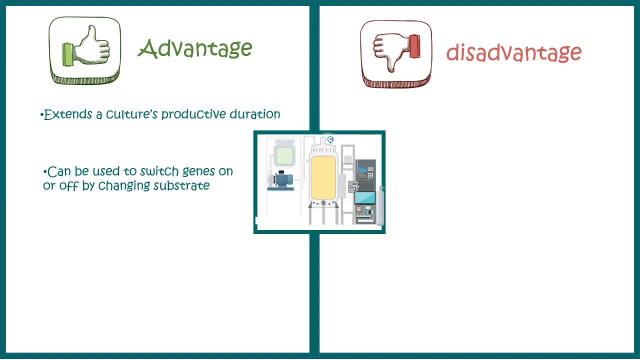 type of bio process, Let's say, which requires periodic switching on and switching off of a gene or operon. So in those cases, fed batch process is very good. Now it can be manipulated for maximum productivity using different feeding strategies, So you can modulate the feeding strategies to optimize this process. But the problem 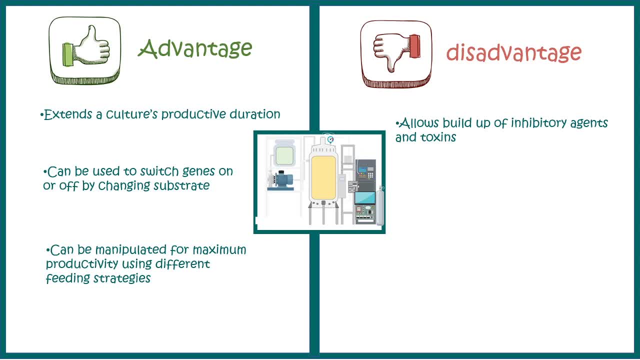 is. though it is better than our batch process, it still allows the buildup of inhibitory agents and toxins. Now it may produce high cell density, which might cause a problem in downstream processing and other cases. So there are disadvantages to this process as well, But we should also focus. 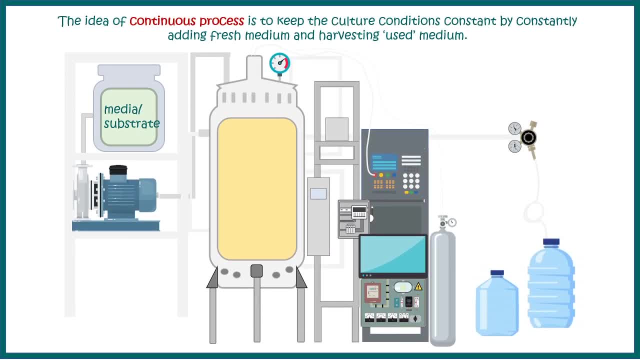 on the added advantages. next we'll talk about that continuous process. The idea behind continuous process is to keep the culture conditions constant By creation, routine processes and natural technology we can forgot about. the Last one is culture and processes. To add Shiva's jaotica in two additional decisions causes. 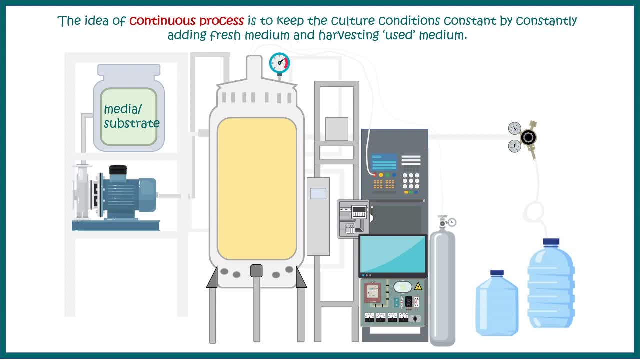 always adding fresh medium and harvesting the used medium. so here we would understand the process of steady state. so here you would have a media reservoir or substrate reservoir, from where you can give sequential input over time and you would have a sequential outlet, like you can take out the products which would have your cells and media. 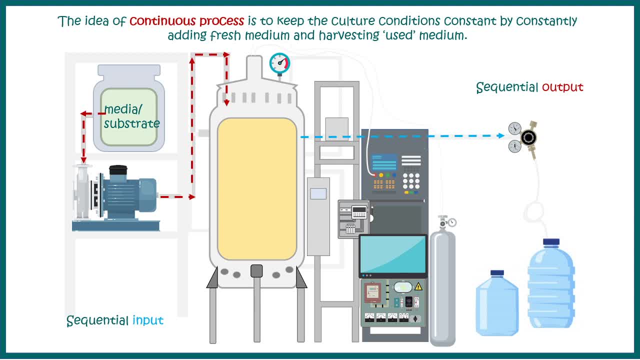 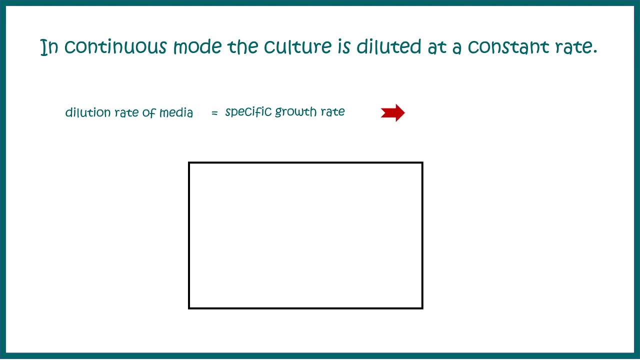 you can take it out in different point of time. so sequential input and sequential output is the key feature of continuous process. moreover, in continuous process, the dilution rate of the media is exactly equal to the specific growth rate, and that tells us that cell density, or the viable cell density, remains constant throughout this process. and that's the biggest. 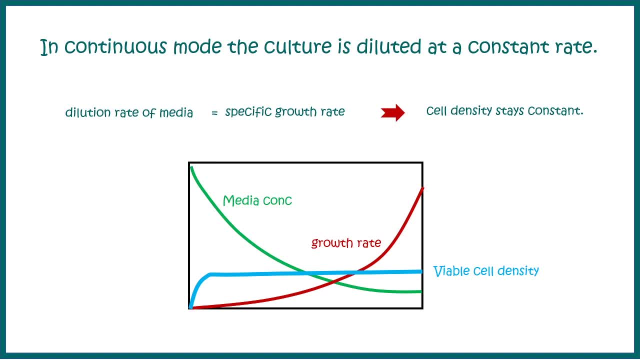 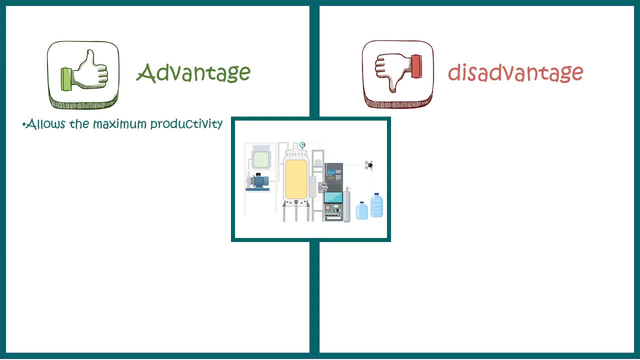 advantage of continuous process. In modern day industry they are really adapting this continuous processes over fed, batch or batch processes. the advantage we have already kind of discussed that it allows maximum productivity because reaction downtime is low and you don't have to shut down the reactor after every run. 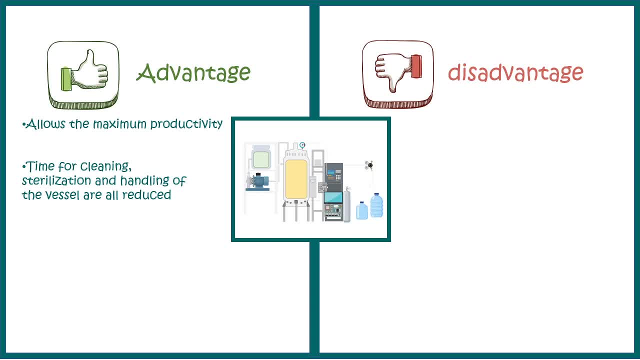 so the time for cleaning, sterilization, all of these aspects which can delay the whole process or reduce the effective time, is minimized using a continuous bio process. lastly, it provides a steady state for metabolic studies. so if you are especially doing metabolic studies in industry or trying to make or purify some metabolites, this kind of processes would be very useful. 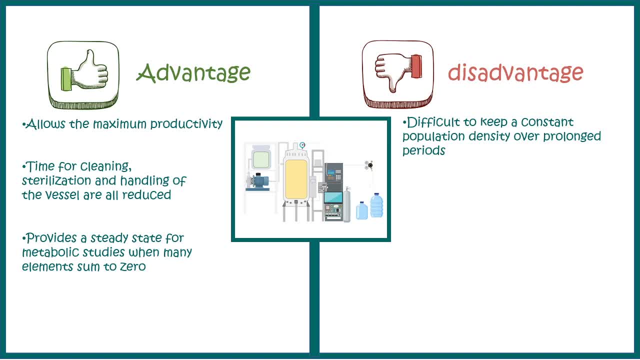 now, though theoretically it looks very advantageous, but the difficulty is to keep a constant population of viable cells right, so this is practically difficult. okay, the products of a continuous process cannot be neatly separated into batches, so traceability is difficult. maybe one in batch process, maybe one batch was not good, you can discard that batch, but here if the whole run.